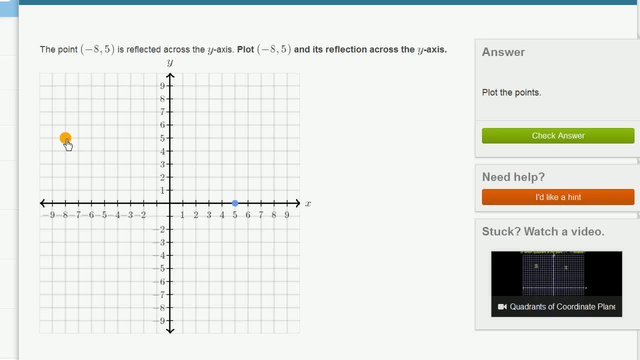 So we've plotted. Now we have to plot its reflection across the y-axis. So you can imagine if this was some type of lake or something and you were to see its reflection, and this is say, like the moon, you would see its reflection roughly around here. 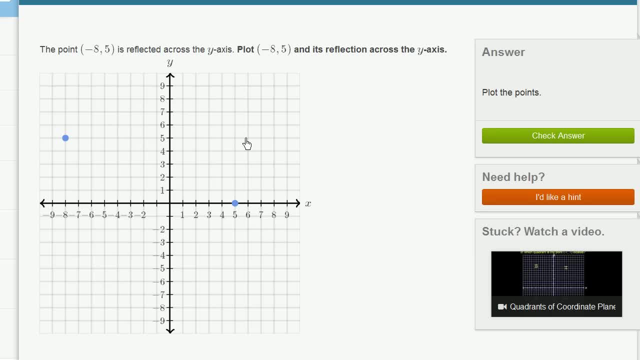 You would see an equal distance away from the y-axis. So you would see it. You would see it at 8, to the right of the y-axis, which would be at positive 8, and still 5 above the x-axis. So that's its reflection right over here. 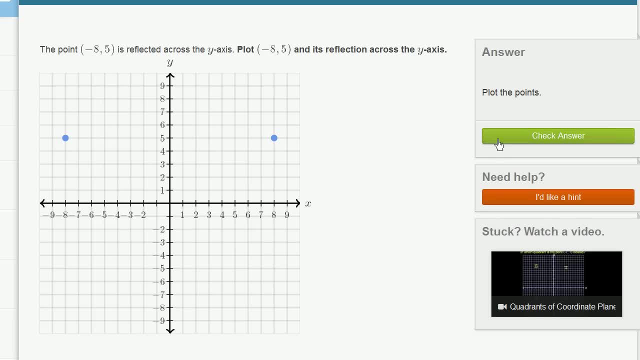 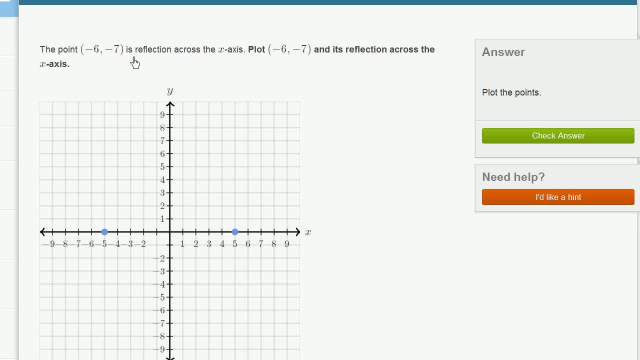 Its reflection is the point. Let's do a couple more of these. The point is reflected across the x-axis Plot and its reflection across the y-axis. So we're going to go 6 to the left of the origin and we're going to go 6 below and we're going to go down 7.. 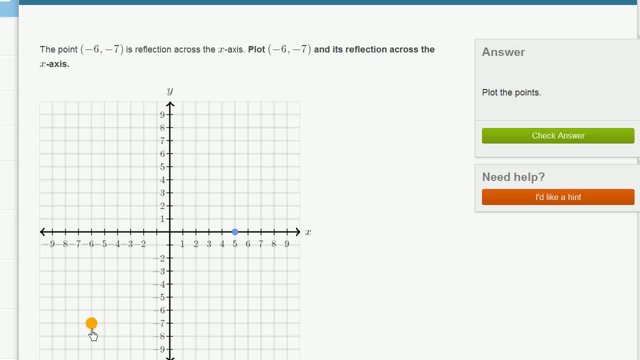 So there we go is right there, And we are reflecting across the x-axis. So, once again, if you imagine that this is some type of a lake, or maybe some type of an upside-down lake or a mirror, where would we think we see its reflection? 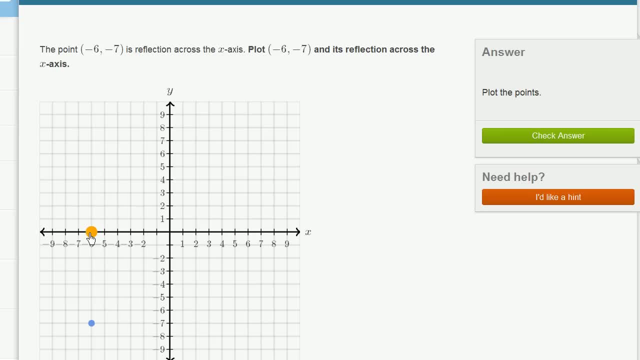 Well, its reflection would be the same distance. We're reflecting across the x-axis. So it would be the same distance, but now above the x-axis. So this was 7 below. Now we're going to go 7 above the x-axis. 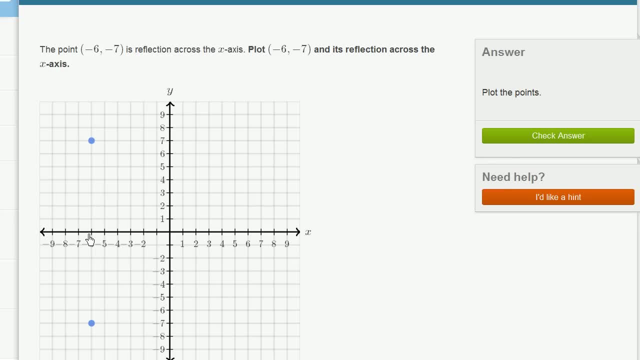 and it's going to be at the same x-coordinate. So there you have it right over here. We reflected this point to right up here because we reflected across the x-axis. Let's check our answer. Let's do one more. The point is a reflection of point. 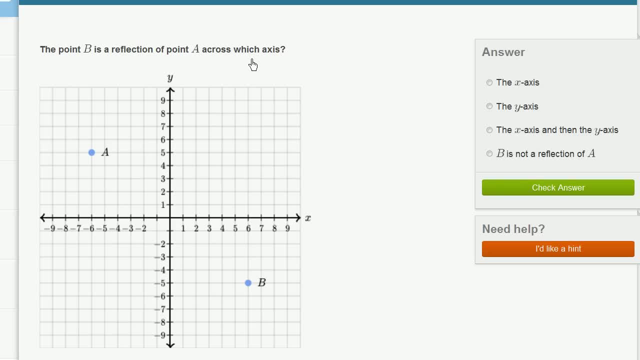 Reflection of point. across which axis? So let's think about this right over here. This is at the point. This is at the point. So let's see It doesn't look like it's only one axis If I were to reflect this point across the y-axis. 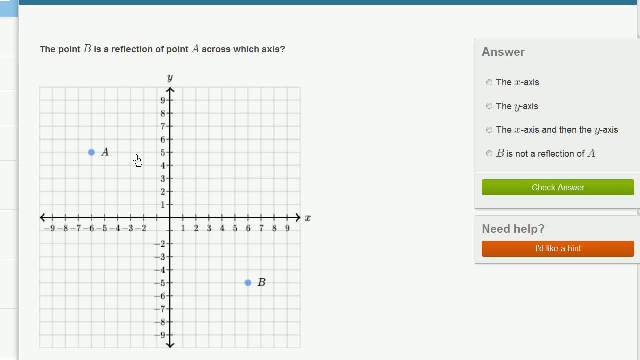 it would go all the way to positive 6, 5.. So it would go all the way right over here. So if I reflect a just across the y-axis, it would go there. And then if I reflect a just across the y-axis, it would go there.